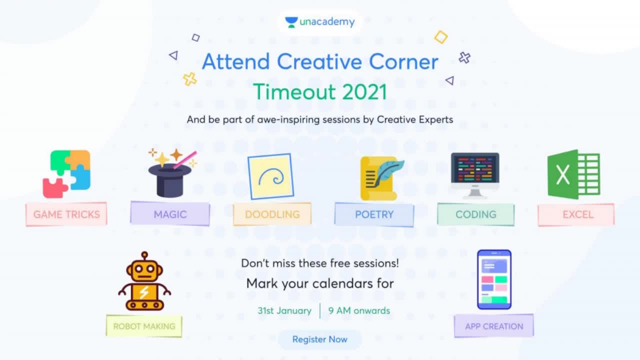 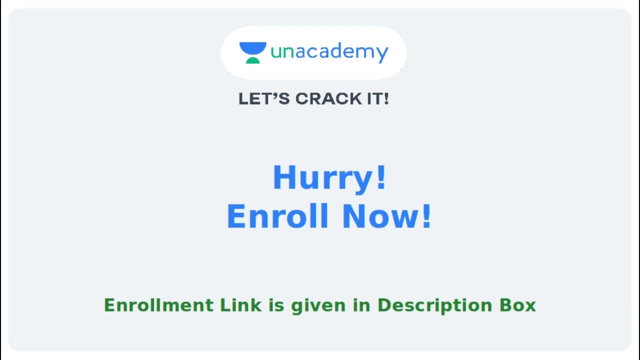 Creative Corner. Timeout is on 31st January 2021.. Sounds interesting. To enrol free for this event, you need to check the enrolment link given in the description box To enrol. you can also download the Unacademy app from the Play Store. 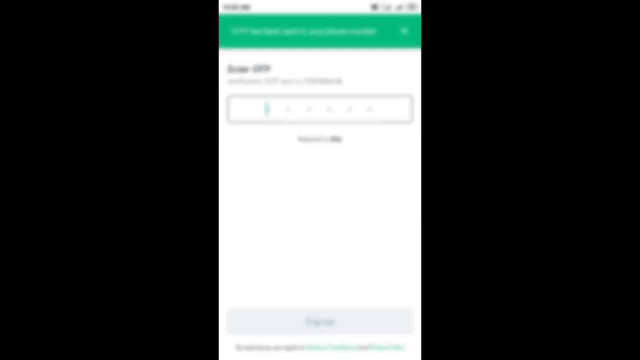 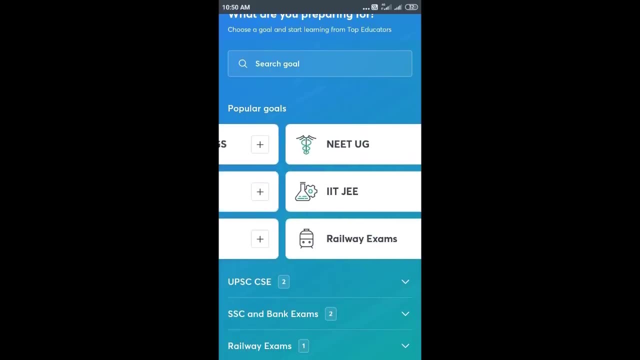 Then enter your mobile number for sign up. Fill all the details, such as your name, email address and your state. By completing this process, you will get an OTP on your mobile number. Just enter the OTP and you will be in an Unacademy family. 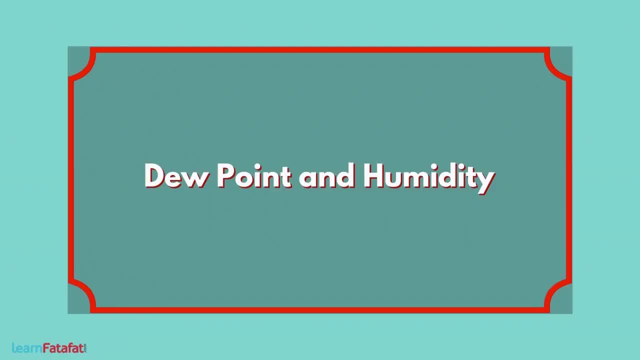 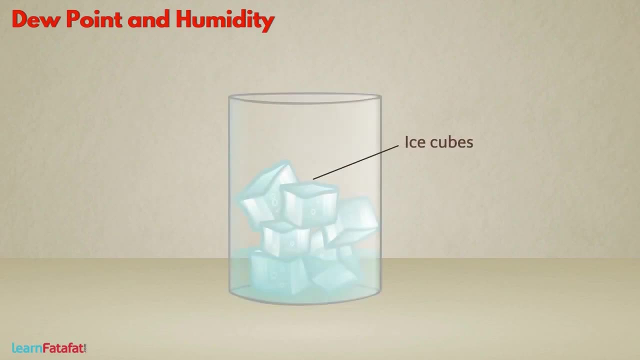 So let's crack it. Dewpoint and Humidity: If you keep few ice cubes in the glass, then after some time you will notice water drops appearing at outer side of the glass. Can you tell me from where these drops appear? Do water flow from inside of glass to outside? 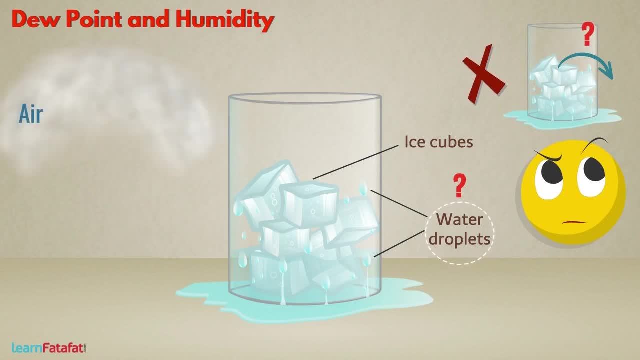 No, We know that air is a mixture of gases, But do you know that air also contains some amount of water vapours? They enter in air as a result of heating of water by solar energy. Air containing water vapours is called moist air. 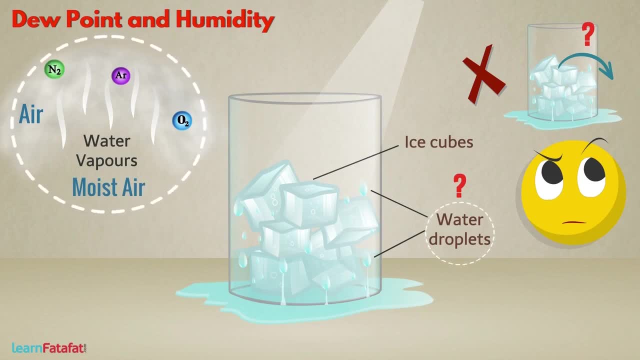 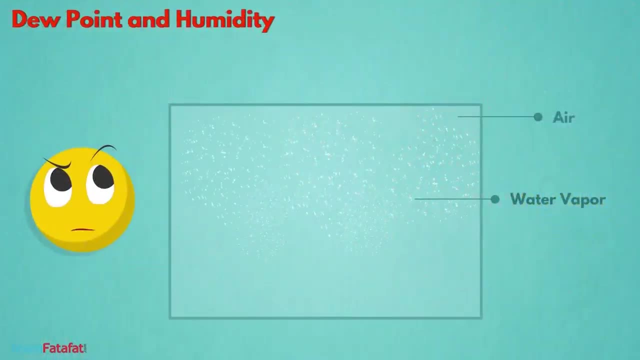 Moist air contains water vapours. The amount of moisture or water vapour present in air is called humidity. What will happen if the amount of water vapours in the given amount of air increases continuously, Basically, at a given temperature, a fixed amount of air. 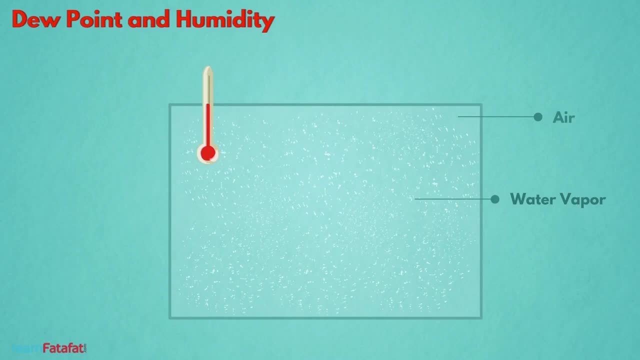 can contain only up to certain maximum amount of water vapours. At this stage, air is said to be saturated with water vapours. If the amount of water vapours is increased beyond this amount, then the excess water vapours undergo condensation. 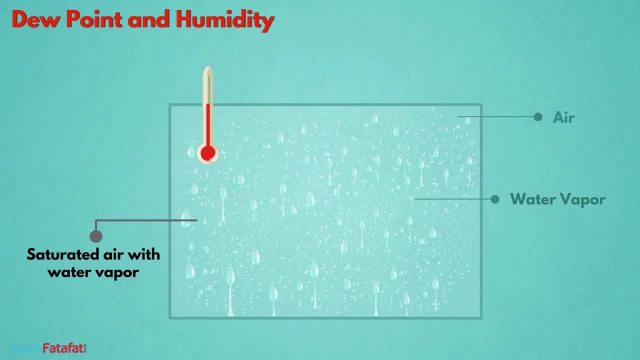 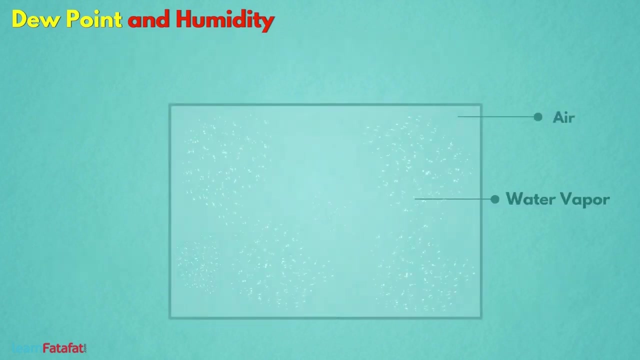 That is, conversion of gas form to liquid form. Thus water vapours get converted back into liquid water. The temperature at which air becomes saturated with vapours is called dewpoint temperature, or simply dewpoint, A given amount of air which contains less amount of vapours than maximum.